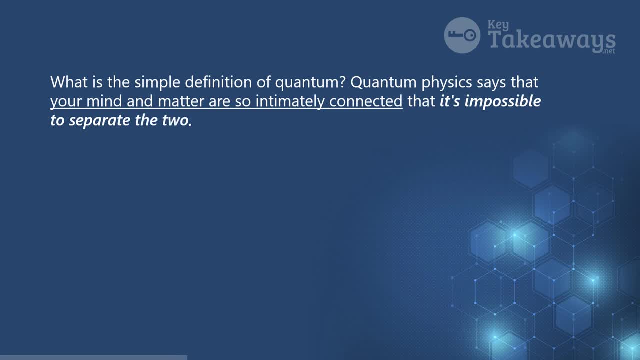 that it's impossible to separate the two. That matter has a mind and mind is a matter, And you can't pull them apart. And so Newtonian physics, the world we live in, is the physics of the predictable. Okay, we're going to shoot a rocket to the moon. we need to know the distance, we need to know the speed. 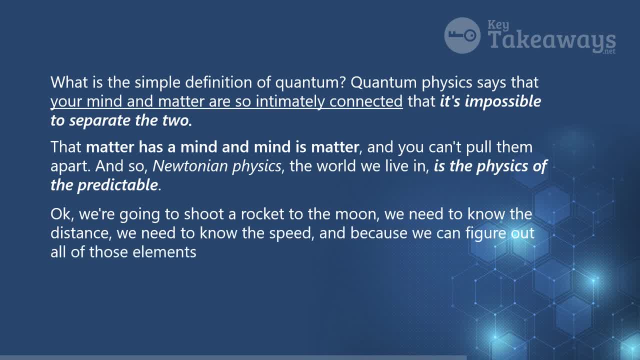 and because we can figure out all of those elements, we could say that Newtonian physics: we can predict the future, We can predict where we're going, We can predict how much time it takes, But the quantum model of reality is about the unpredictable. 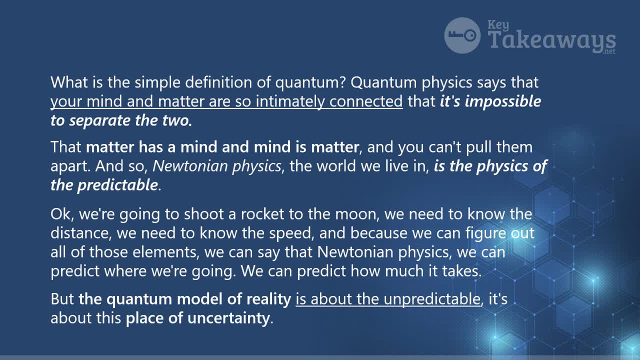 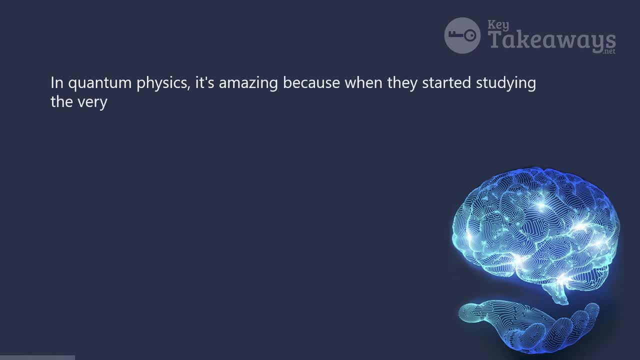 It's about this place of uncertainty, And so in quantum physics it's amazing, because when they started studying the very tiny particles in atoms like electrons and photons, they expected that those particles would behave like planets, Like planets rotating around the sun. 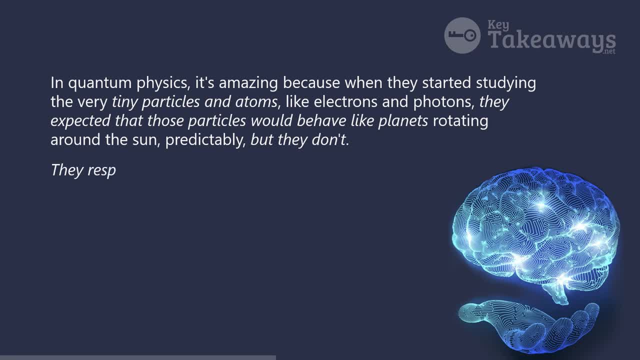 Predictably, But they don't. They respond to mind. And so now, all of a sudden, the quantum physicist comes along to measure the electron, And the electron goes from a wave of possibility, and all that energy collapses into a particle. 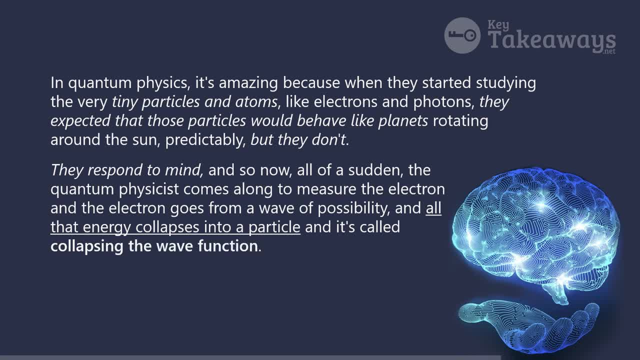 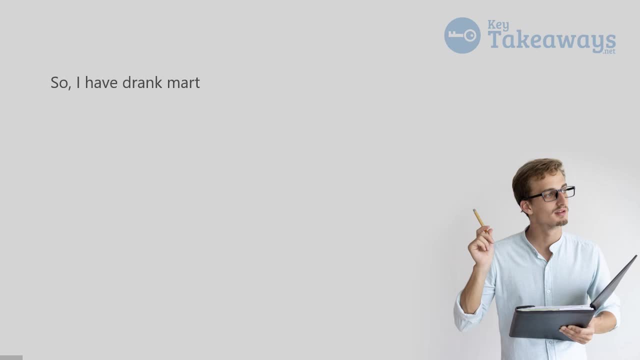 And it's called collapsing the wave function. They turn their back and no longer look and observe the electron And it turns back into energy. So mind is affecting matter. So I have drank martinis with quantum physicists till sunrise hundreds of times. 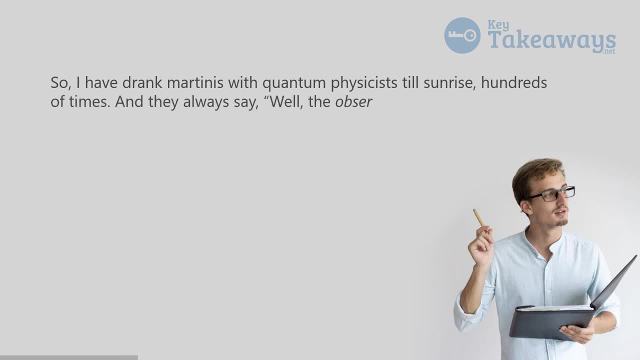 And they always say: well, the observer effect works really well for the tiny, small subatomic particles, but not for the very large. And I always say the same thing to them: Yeah, the observer does work for the very tiny and not for the very large. 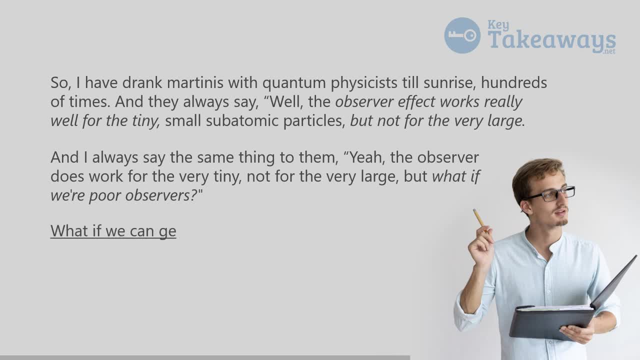 But what if we're poor observers? What if we can get better at observation? In other words, if you wake up every morning and you do the same thing that you've been doing for the last ten years, then you're caught in the predictable world of Newtonian physics. 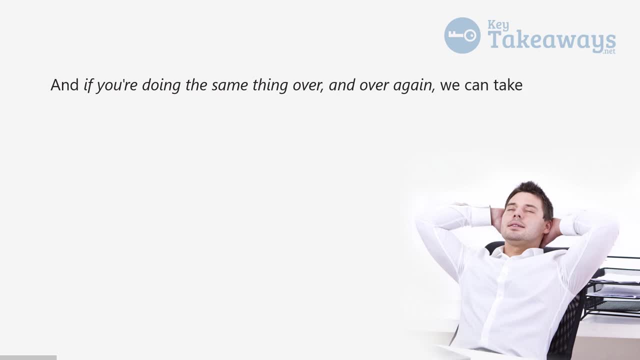 And if you're doing the same thing over and over again, you can take your past and lift it up and set it on your future, and it's going to be exactly the same. So then, if you're viewing your life from the same level of mind every single day, 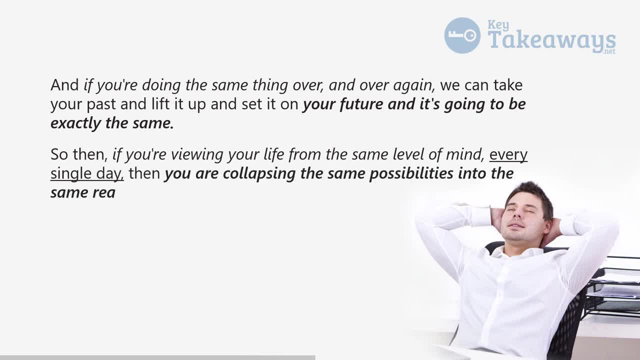 then you are collapsing the same possibilities into the same reality. So if you teach people then to find the present moment, In quantum physics all possibilities exist in the present moment, But most people's brains are anticipating the future based on the past. 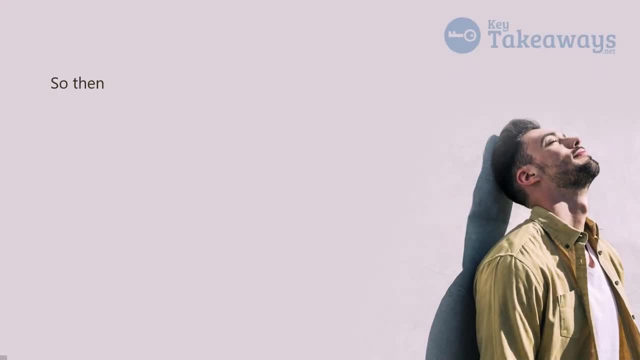 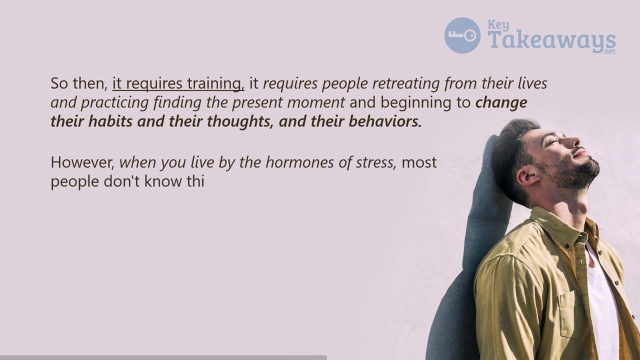 and they're not present. So, then, it requires training, It requires people retreating from their lives and practicing, finding the present moment and beginning to change their habits and their thoughts and their behaviors. However, when you live by the hormones of stress, most people don't know this. 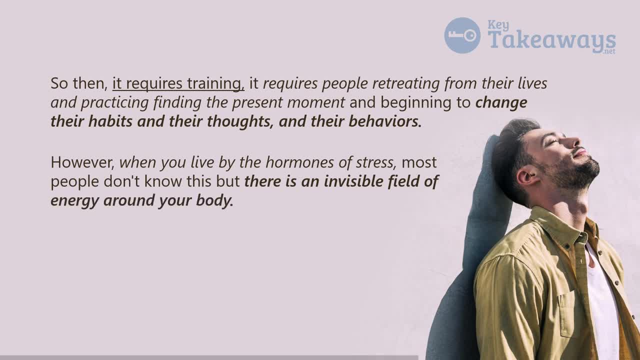 but there's an invisible field of energy around your body And when you react to someone or something, you draw from this invisible field and you turn it into chemistry And the field around your body shrinks. How do I know? I measured it. 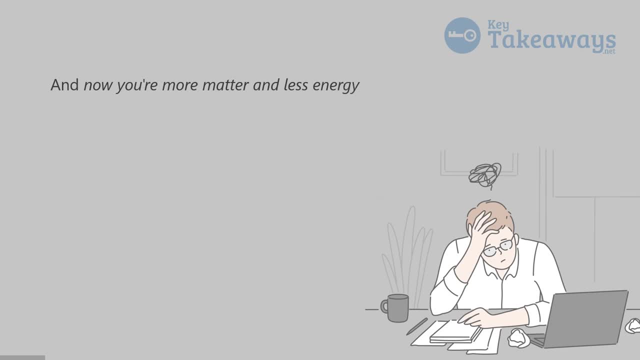 And now you're more matter and less energy, You're more particle and less wave, And most people then, when you are matter, trying to change matter, you always try to force the outcome, You try to control the outcome, You try to predict the outcome. 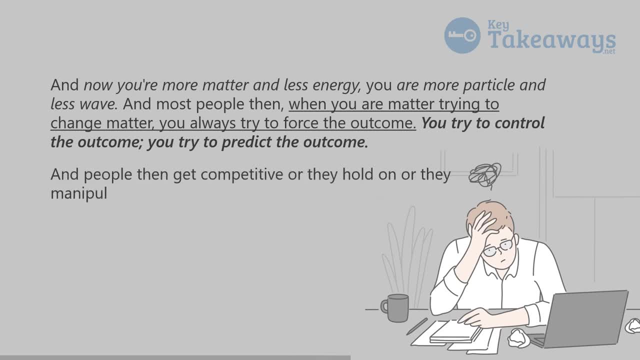 And people then get competitive, or they hold on, or they manipulate, or they cheat or they steal, because that's the only way they can get what they want. But the quantum model of reality, when you are truly in the present moment. 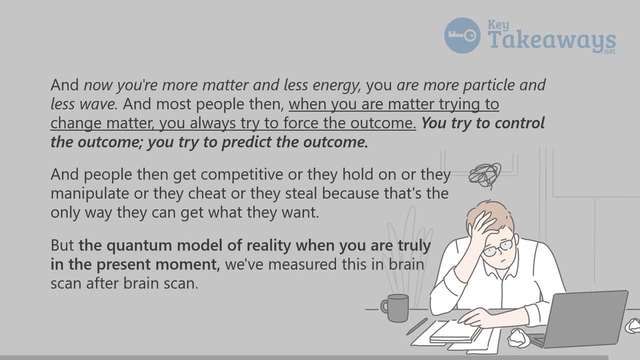 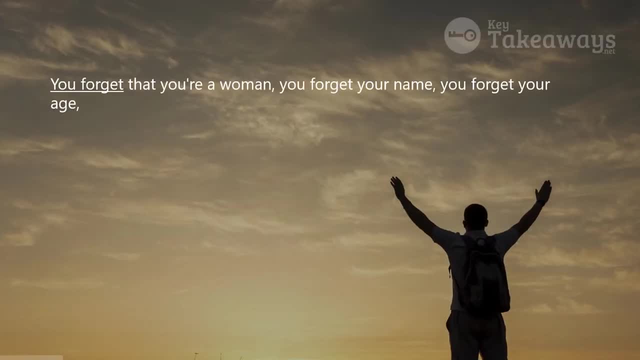 and we've measured this in brain scan after brain scan. you forget that you're a woman, You forget your name, You forget your age, You forget your culture, You forget your past, You forget your future. You forget that you have a body. 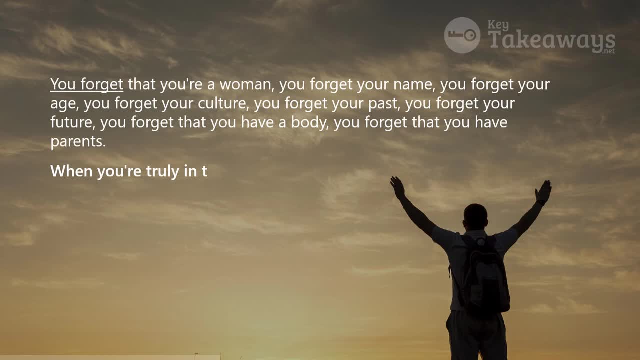 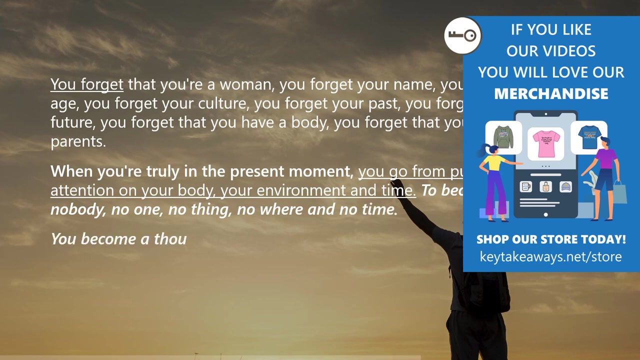 You forget that you have parents When you're truly in the present moment. you go from putting your attention on your body, your environment and time to becoming nobody One, no thing, nowhere, in no time. You become a thought alone in possibility. 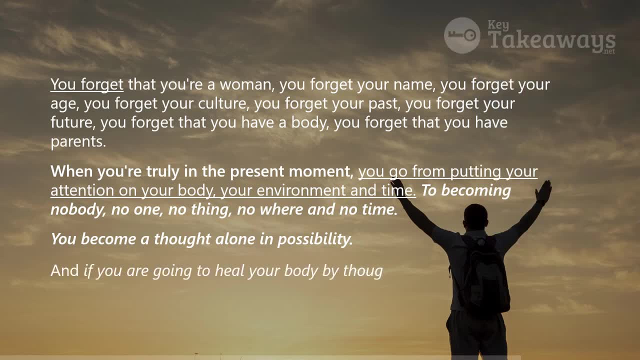 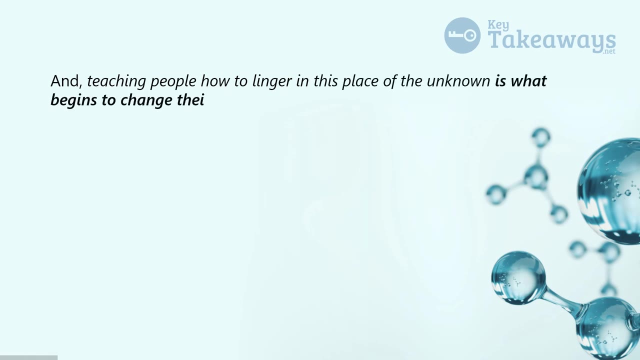 And if you are going to heal your body by thought alone or change something in your life by thought alone, then you have to become thought alone, And teaching people how to linger in this place of the unknown is what begins to change their energy. 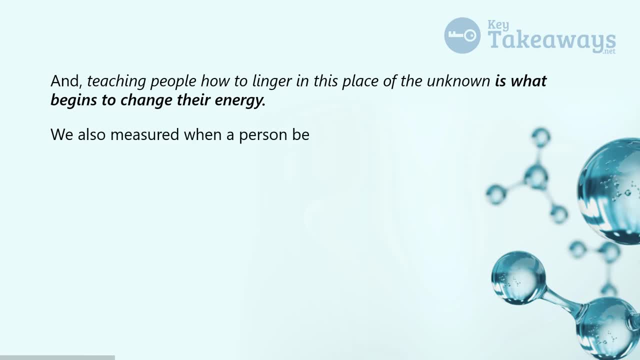 We also measured. when a person begins to open their heart and they can begin to sustain an elevated emotion, They begin to broaden the magnetic field around their body to nine meters wide. Now they're more energy than matter. They're more wave than particle. 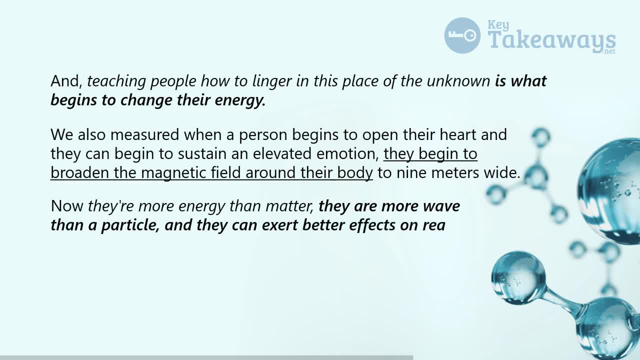 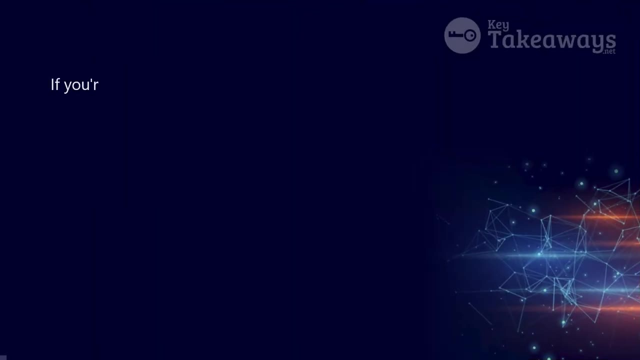 And they can exert better effects on reality. So then, think of when you open your heart. this is science. like dropping a pebble in water: you produce a ripple. If you drop a bigger stone, you produce a bigger ripple If you're able to sustain that state. 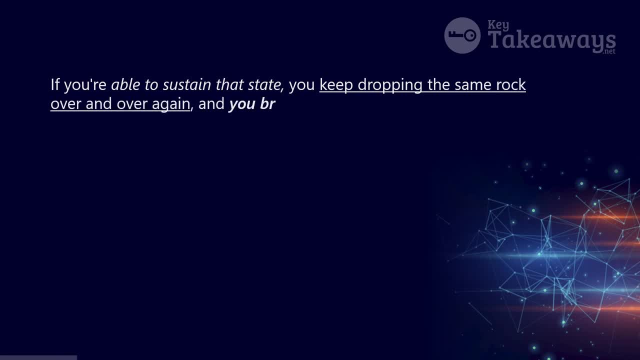 you keep dropping the same rock over and over again and you broadcast a signature into the field. The emotion is the magnetic charge. Your intention, your thought is the information that's carried on that wave. And when you combine a clear intention with an elevated emotion, 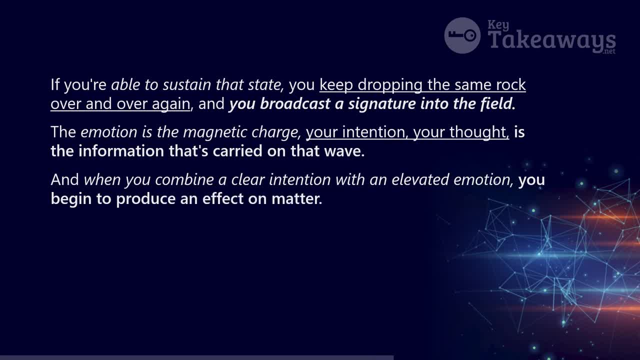 you begin to produce an effect on matter. You see, the thoughts that you think are the electrical charge in the quantum field, The feelings that you emote are the magnetic charge in the quantum field, And how you think and how you feel broadcasts an electromagnetic signature. 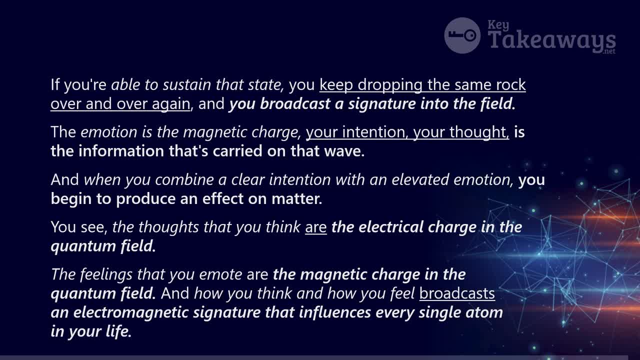 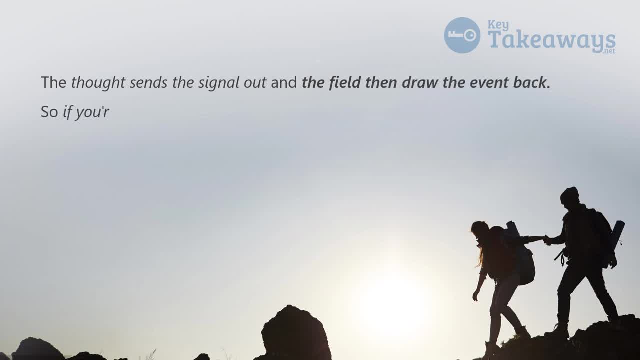 that influences every single atom in your life. The thought sends the signal out and the feeling draws the event back. So if you're walking around your life feeling sorry for yourself and feeling like a victim, you are broadcasting that signature into the field.